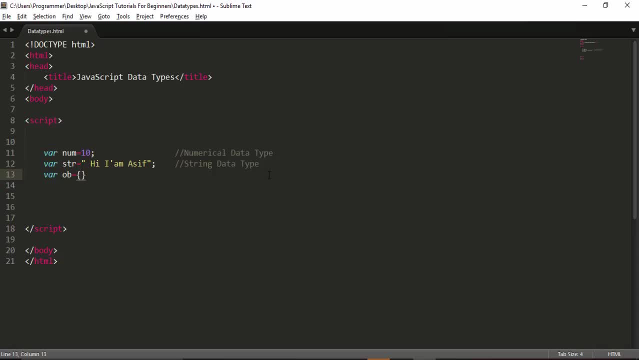 sign in script brackets and I use the type or name and then you need to write the name. for example, I write the first name And I use the colon, and then I assign the value of this variable or this object. I assign the first name, asif, and I use comma. if I will make another object, so I use comma. 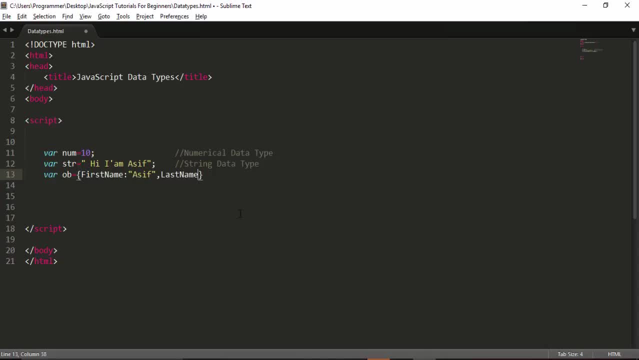 and I use same process, last name, and I use comma, colon and assign the value of this variable. Ok, And finally, you need to write the terminator sign. it is called object, right guys. object, Right guys. we have used three data types: string, or sorry, numerical or integer string and. 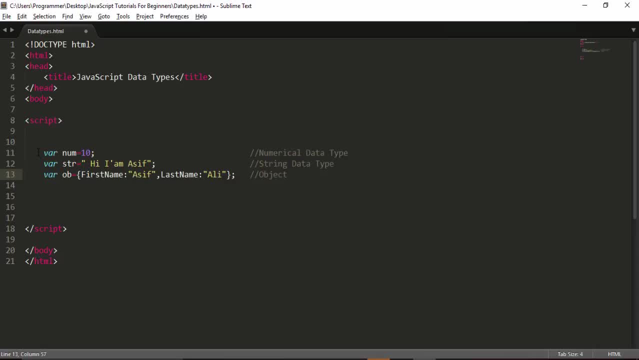 also object. You can use them to perform the operations like insert, update, delete. Yeah, You can use them to perform many other operations- fetching data, store values, and many perform the operation. Right guys, I hope you have understood as well about the variables data types. 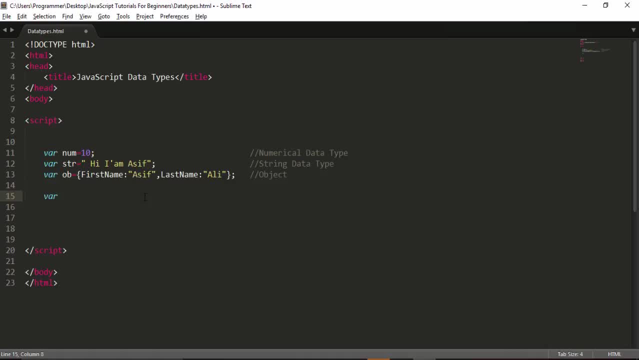 Sorry guys. Now the next thing you need to know. for example, I make a variable blank and I use terminator sign. This is called you have a variable blank. This is called you have a variable blank. This is called you have a variable blank. 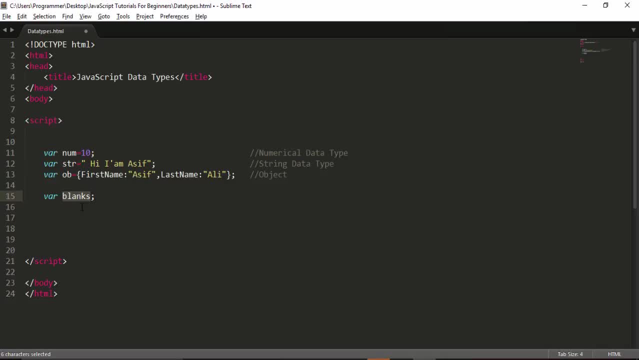 We have. we have made the variable. only we have made the variable. We don't use it. We will use them on letter. How you can use them? That is very simple. For example, you just call the variable name and assign the value on letter.